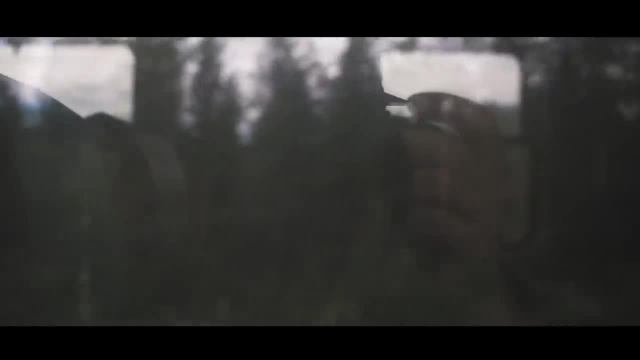 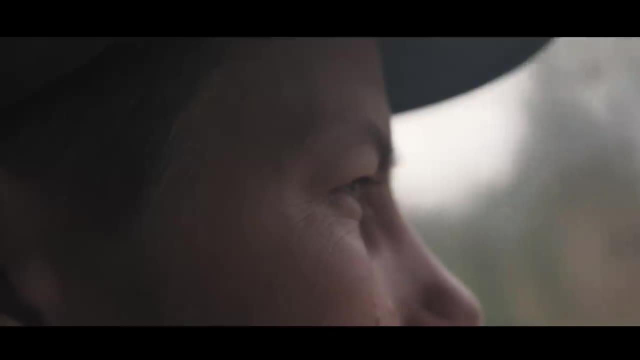 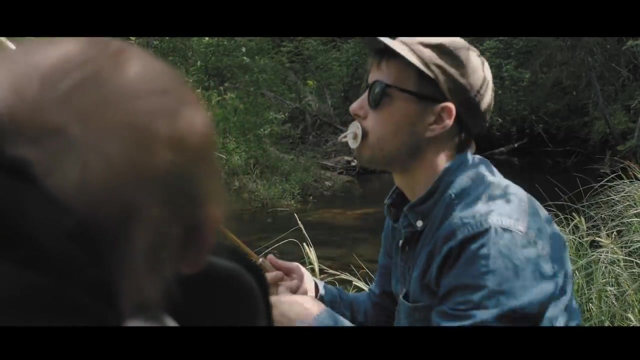 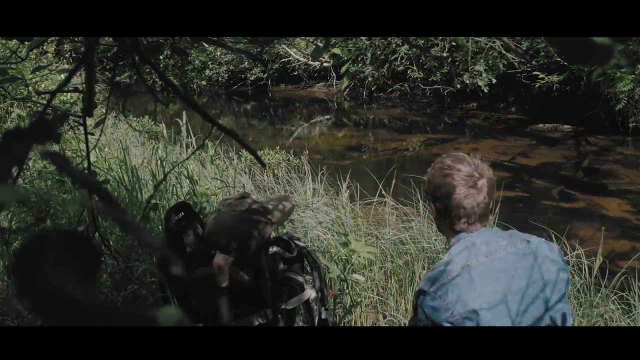 I had just turned 30 and I was filming myself in slow motion. The recent changes in my life had made it harder to find time for fishing trips, But there's always a rising trout somewhere in my mind and that's fly fishing for me most of the 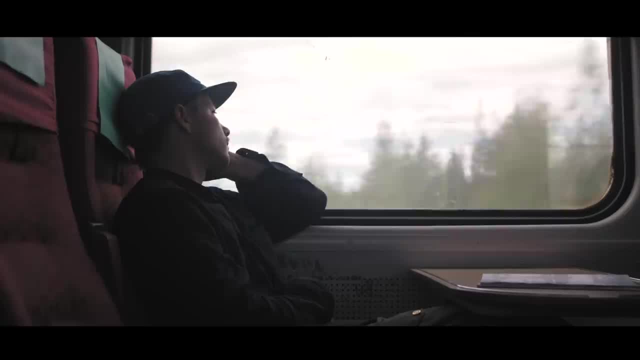 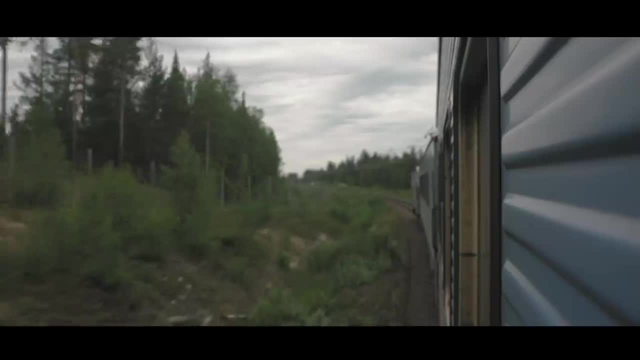 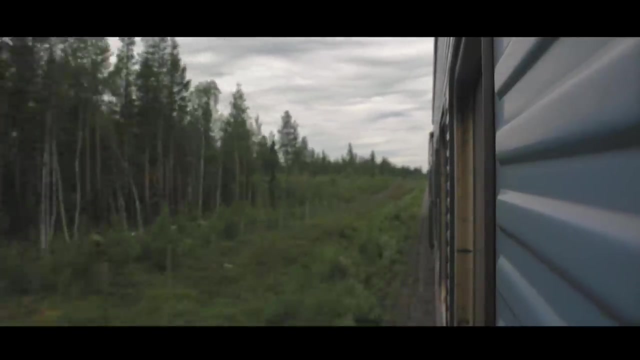 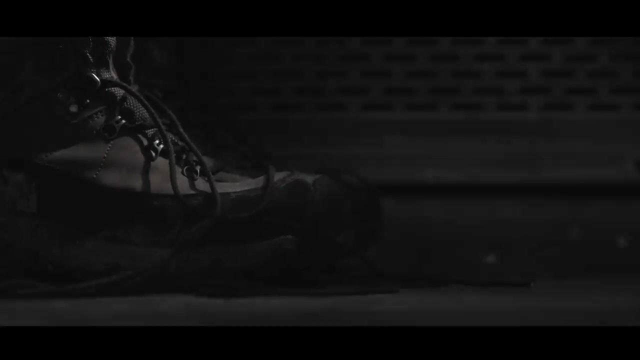 time, The complete opposite of being in the moment. It's this idea of being somewhere else. Sometimes that weird tool gets too strong. I just have to follow it. I was headed north On a fishing trip. I first decided to name after the river. 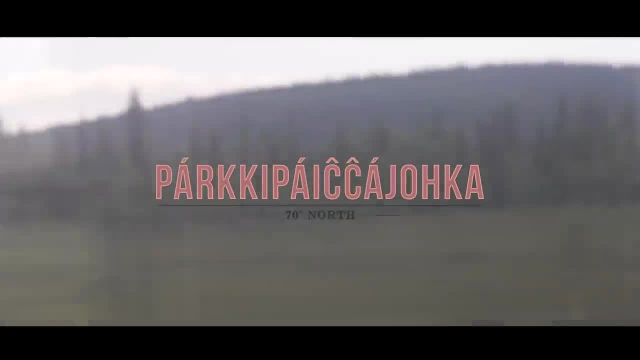 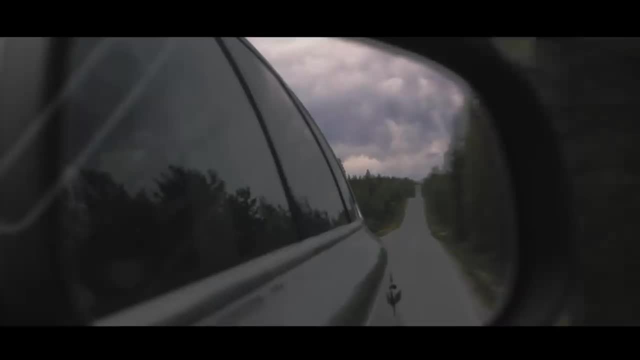 I was headed north On a fishing trip, I first decided to name after the river. I was headed north On a fishing trip. I first decided to name after the river Parki-paika-yoga. When a train couldn't get me any farther, I jumped into a car. 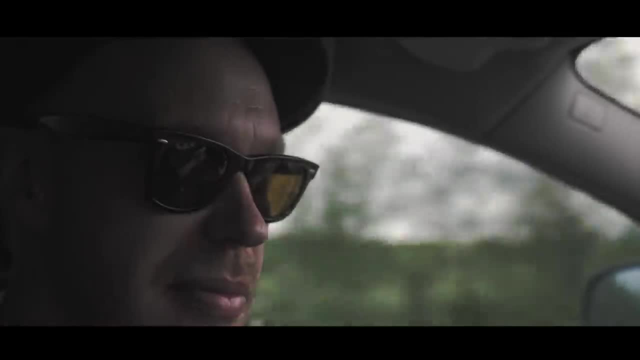 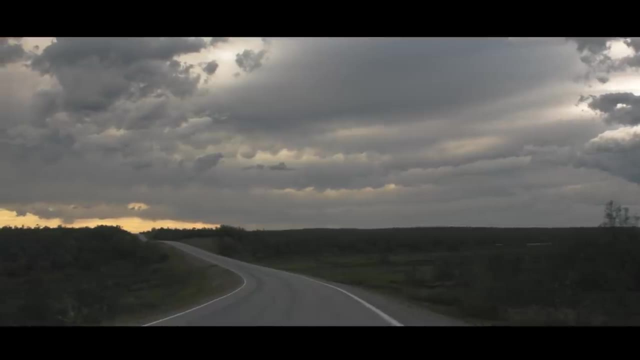 Hold on A jazz musician. I think I considered as a friend at that point of my life was driving us into the barren land north of Sweden. Hold on A jazz musician, I think I considered as a friend at that point of my life was driving us into the barren land north of Sweden. 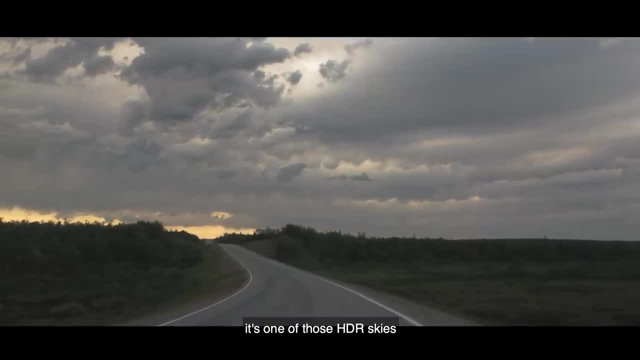 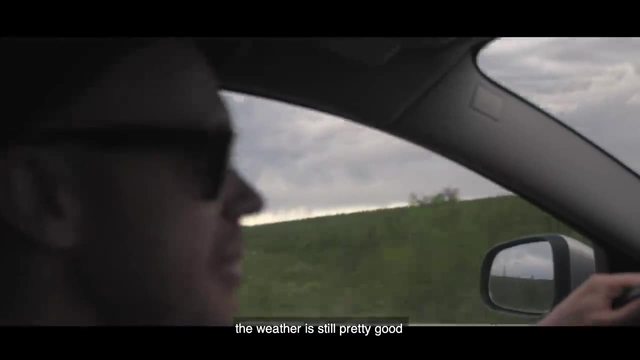 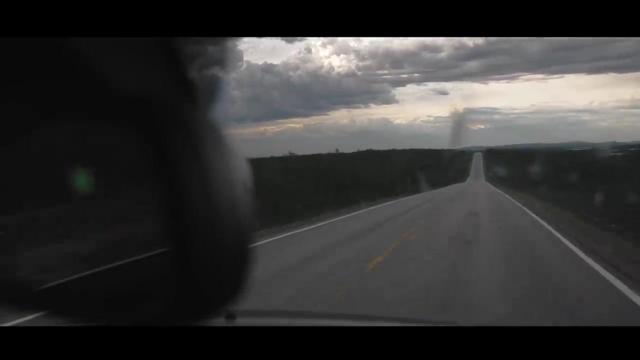 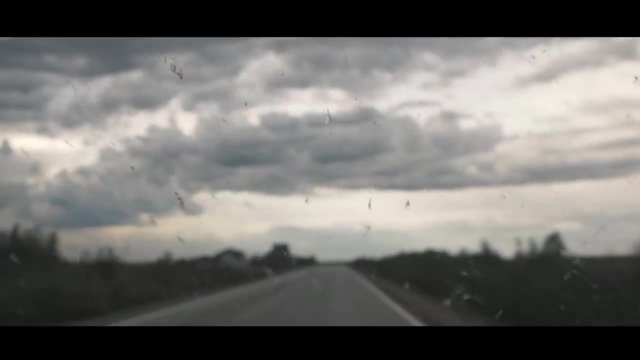 Wow, it's like 2D at the same time. Can you see, it? Is the weather still good, Extremely good. Hovard said he wanted to keep the location a secret, So I renamed the project It was going to be called. 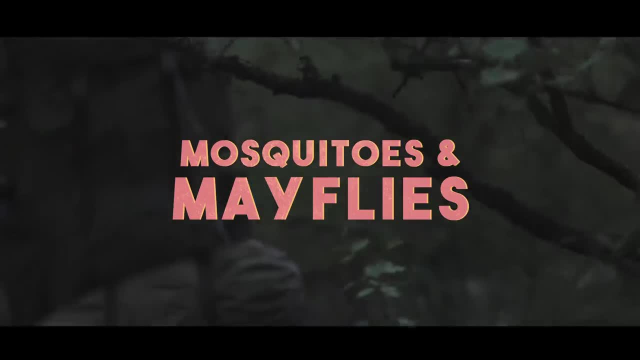 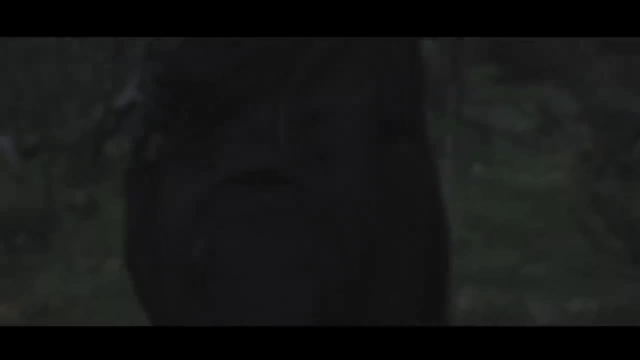 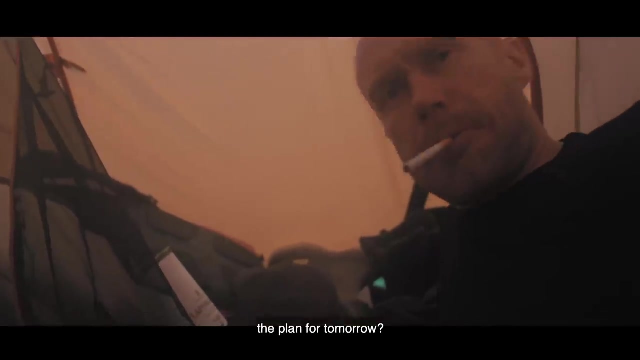 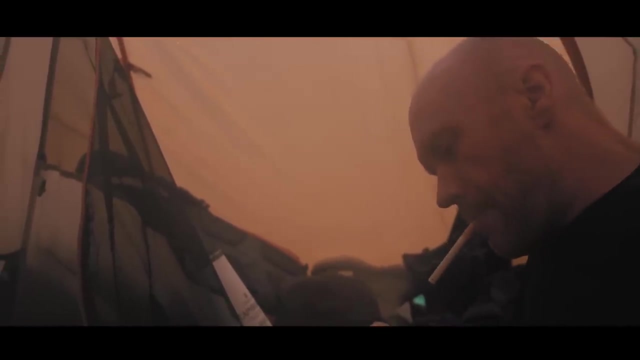 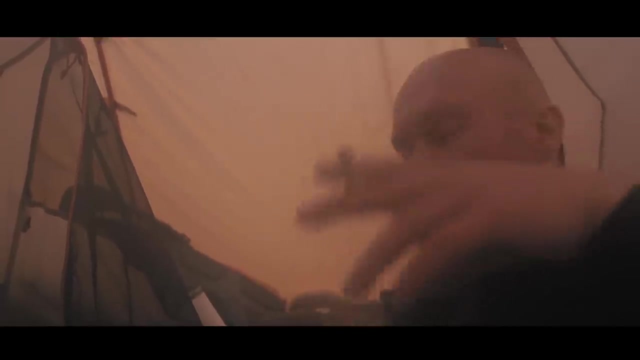 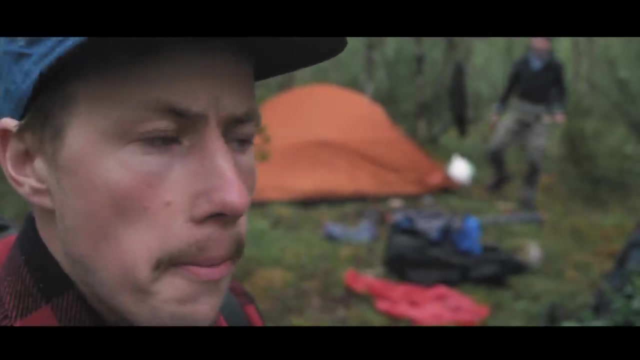 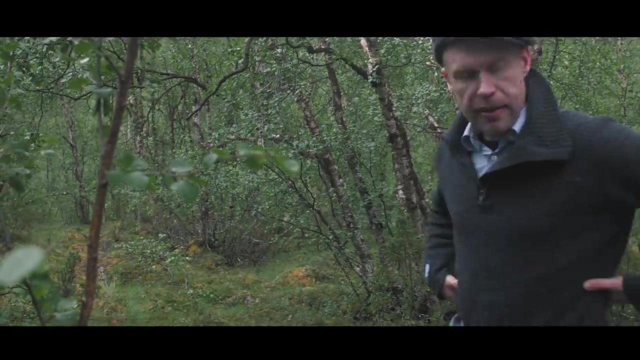 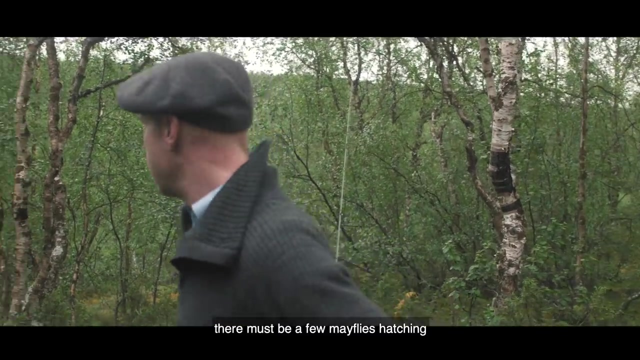 Mosquitoes and Mayflies. No, that's Hopefully. Hopefully it stops raining Sometime. No, it's not a very good situation, but It's getting a little bit better. if you will, A little, thank you. 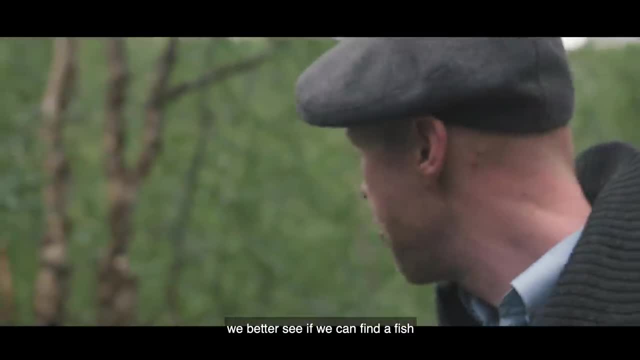 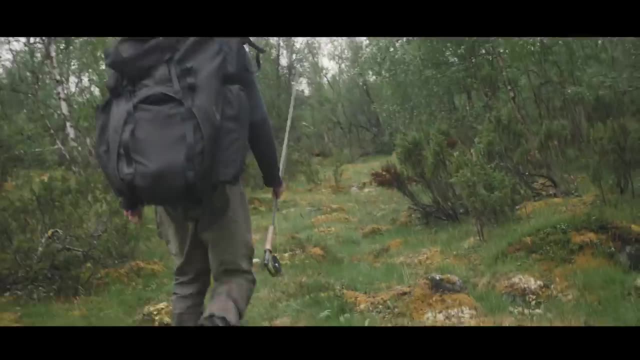 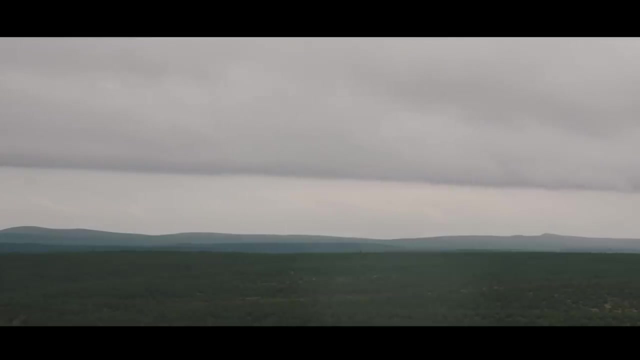 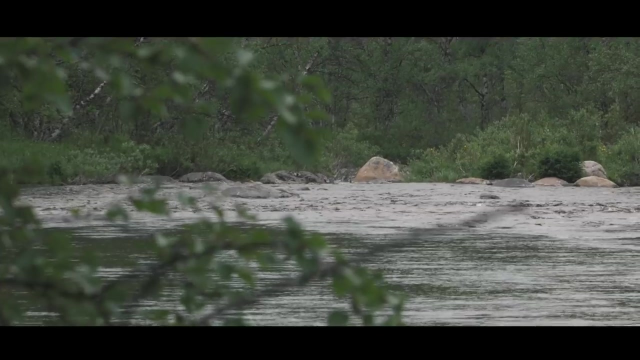 We have to go and see if we can find a fish, Don't you think? I don't think I have much. today It was 14 degrees Celsius, Cloudy And the wind was picking up- Difficult conditions for dry fly fishing. 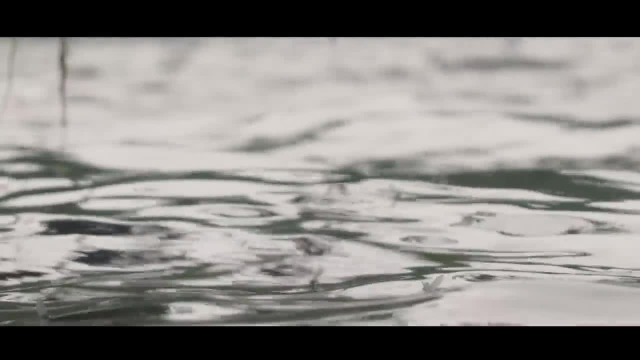 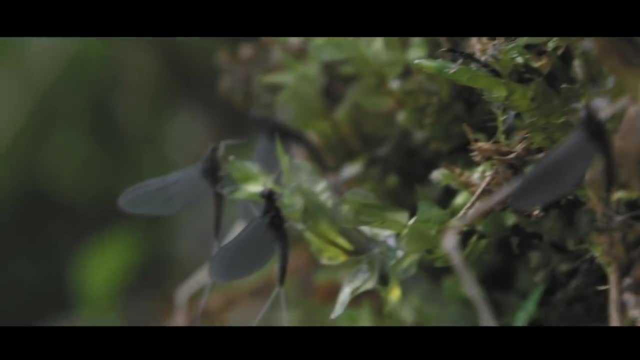 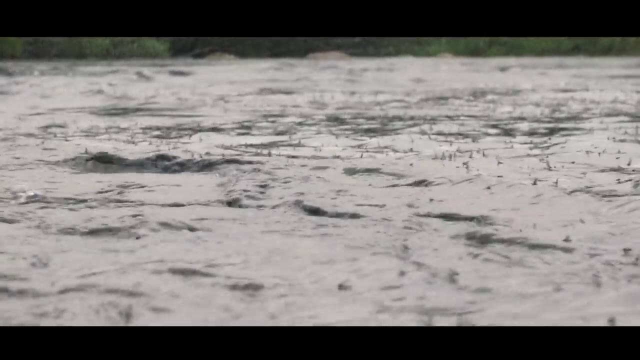 Your only chance is the shit weather. mayfly Beedis rhodana. It's beautiful But very small, And quite often the trout in the river won't really care about the insane number of tiny mayflies on the surface. It's hard to see them. 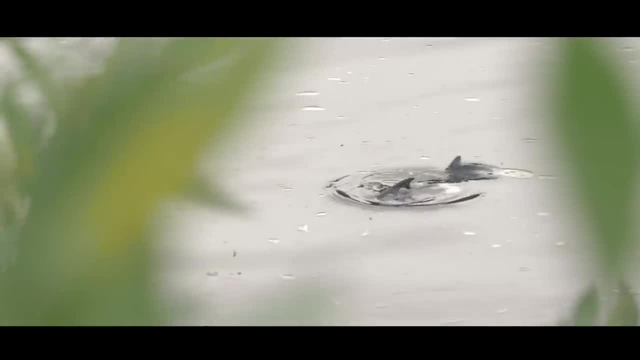 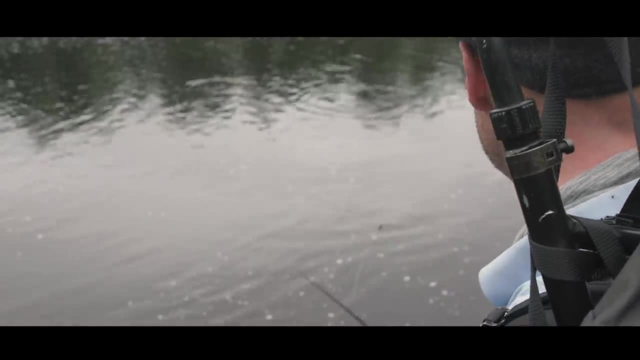 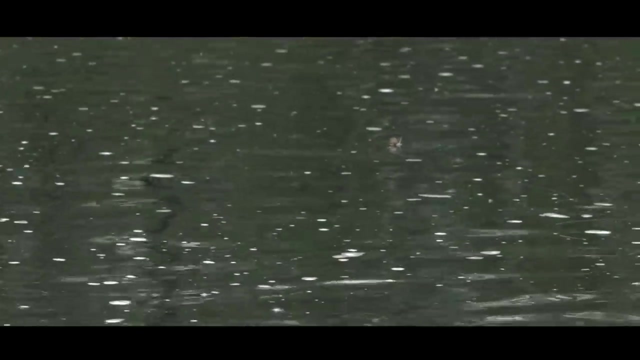 But it's not a big deal. When we finally found the rice, we realized it was the white fish we in Sweden call sik. Can you be fast? You know Fast, Incredibly fast? Okay And fast. Good, You don't spend your time fishing for sik. 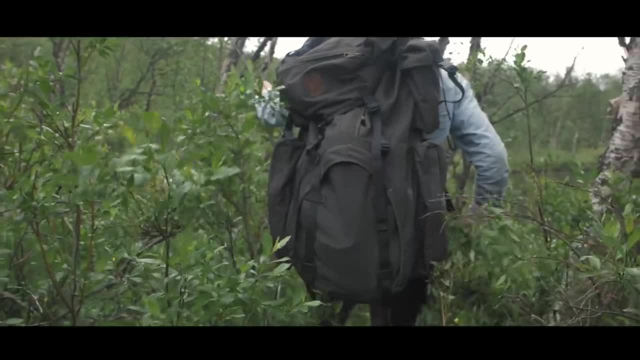 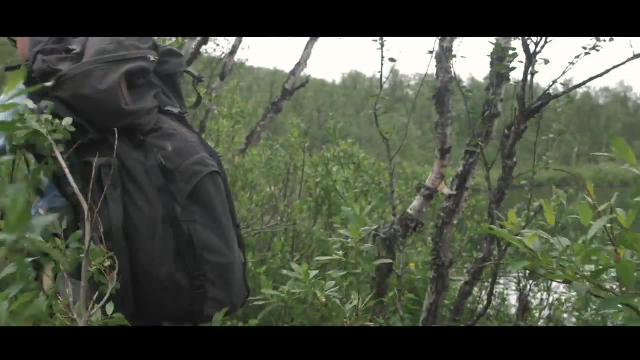 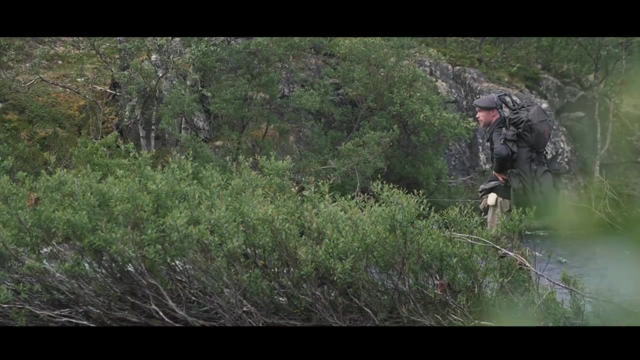 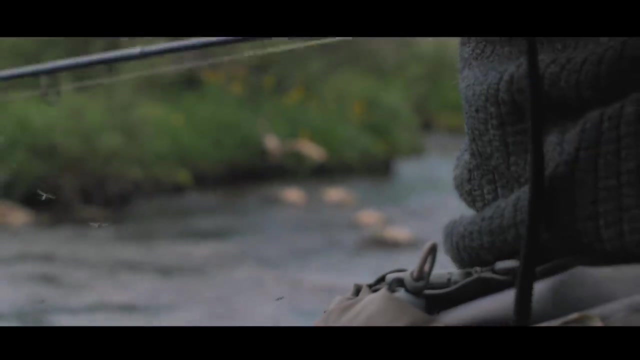 Especially not if you're in northern Finland. No, Hovard had told me many stories about the river And I understood that if we just found one rising trout, there was a big chance it would be the trout of a lifetime. And then 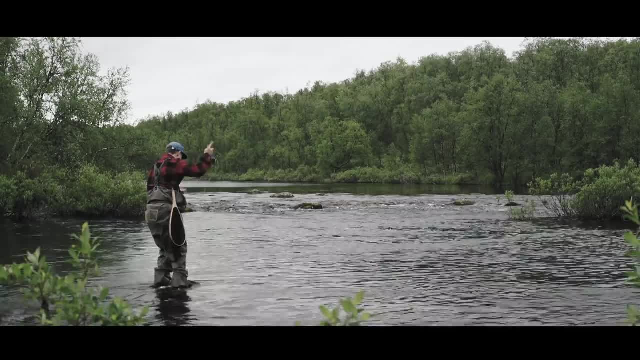 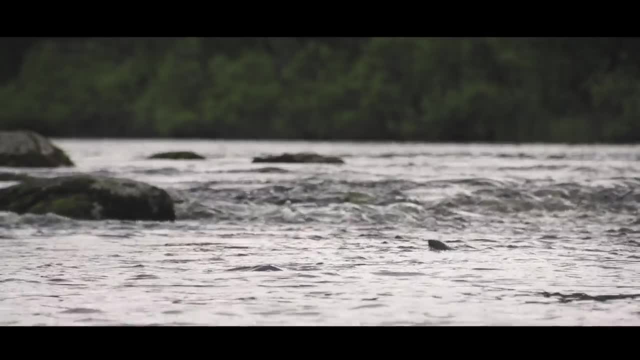 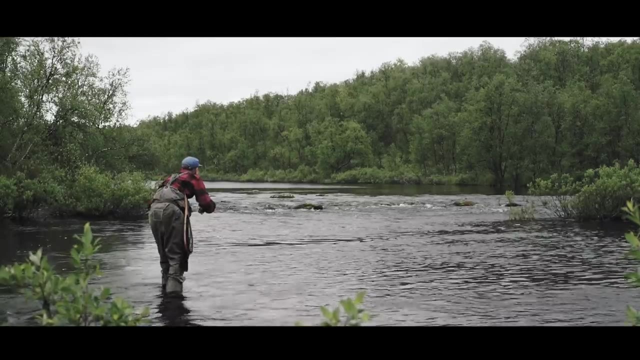 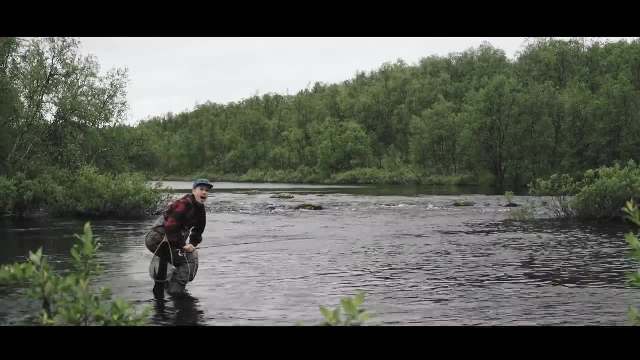 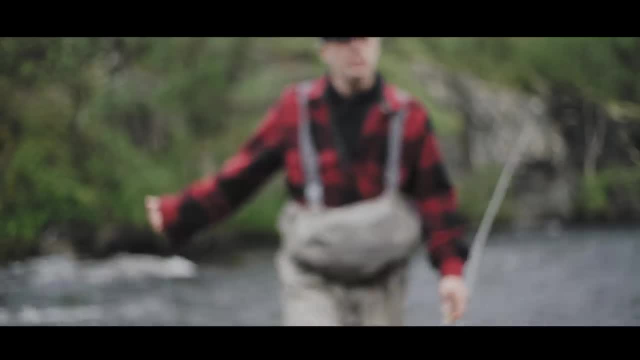 It's a big fish, Yes, And it's big, So we're aiming for a big one That's coming into our eyes. one day They're going to have a big rye trout. It's a big fish, a little bit too good to be true. It's not often I catch a fish that size and 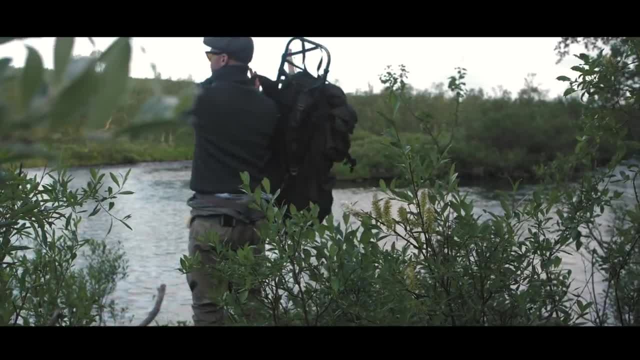 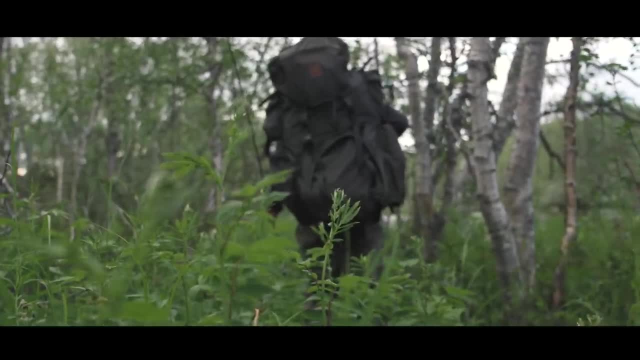 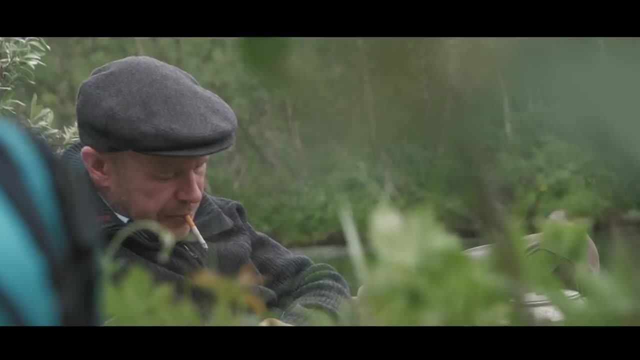 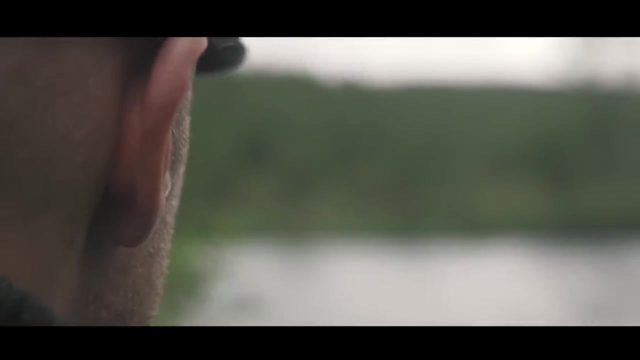 at first I didn't really care that I'd lost it. It was just the first day, But then a few hours passed without finding any more rising fish. I was thinking about what could have been when we got to a place where Hård decided to. 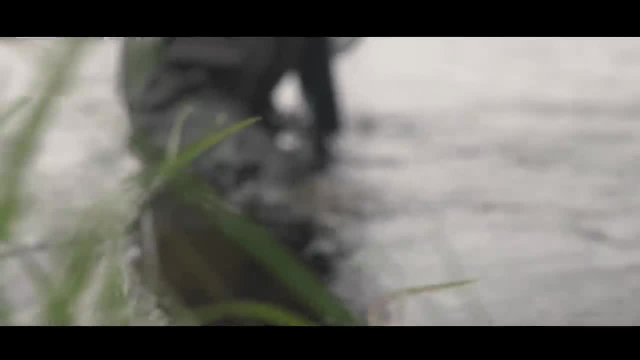 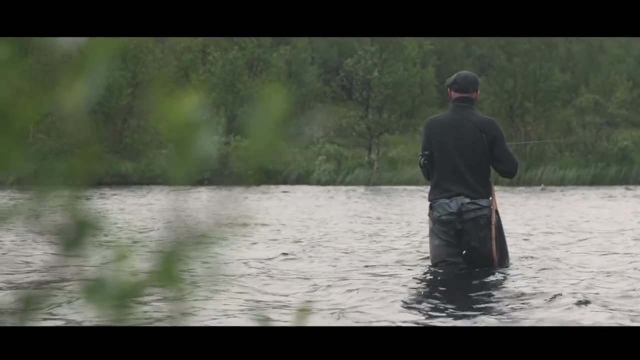 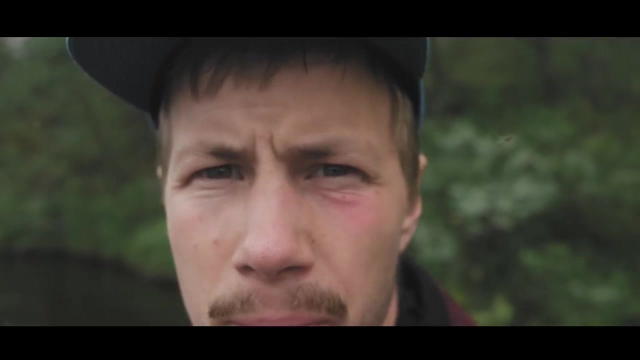 wade out into the stream. We hadn't seen anything. I didn't understand why he was eager to wade out. I stayed on the shore, but as I was filming myself mourning the trout in slow motion while suffering from the first hours of mosquito bites, I 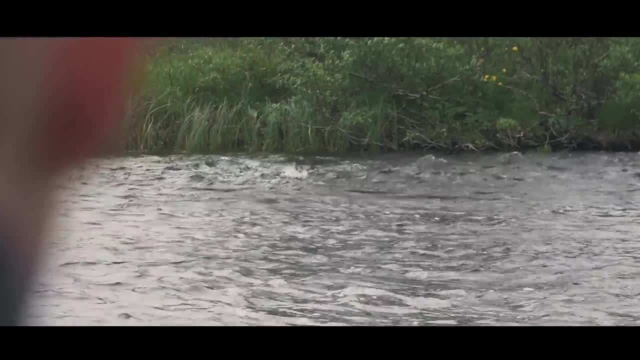 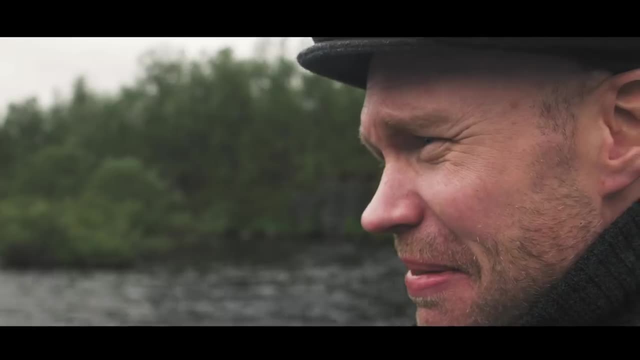 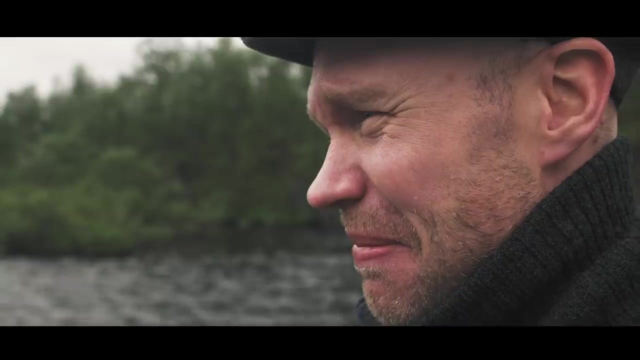 realized he had been here before. He knew this place. Every river have this one place that is a little bit better than the rest of the river. With his back against me, he was wearing a subtle evil smile, And perhaps I went a bit too far when I decided to show him the international symbol of contempt. 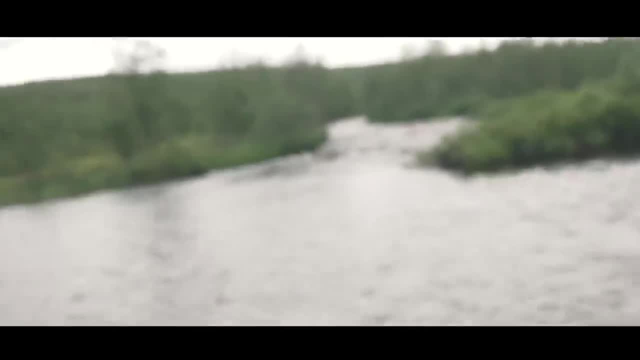 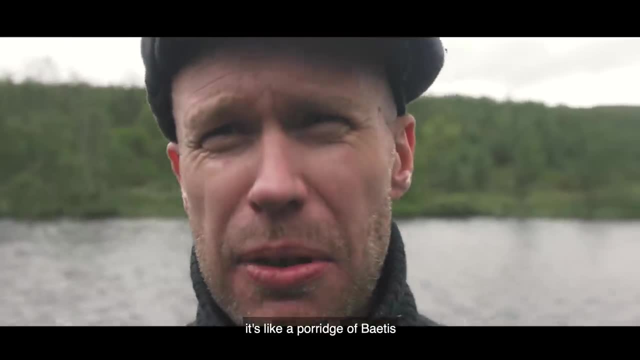 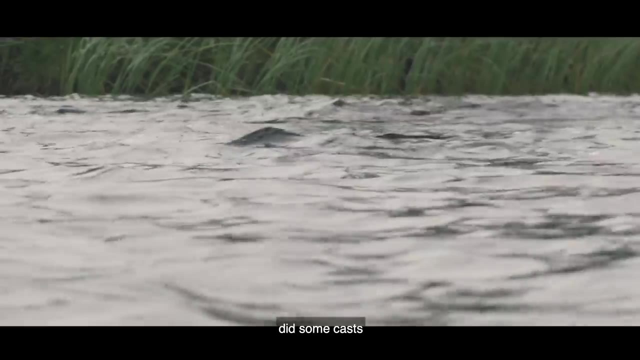 The finger. I was standing up there and you can't see it from here, but it's like a grotto of Baetis out there. But I had a diary on me and when I threw it there was one million Baetis and none behind me. 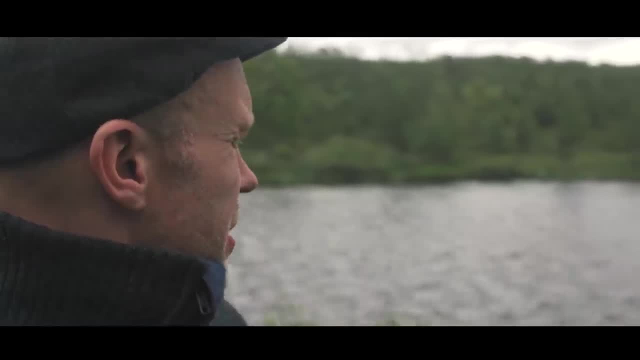 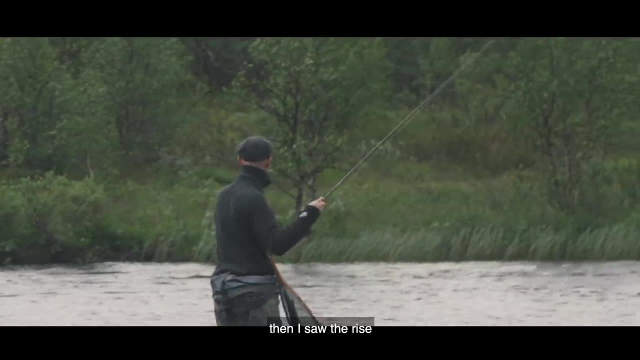 Then I thought I heard something In that side stream And then I heard it again turned around and then I saw what was around me. So I made a few casts of the diary- Nothing- And then I put on my ice cap. 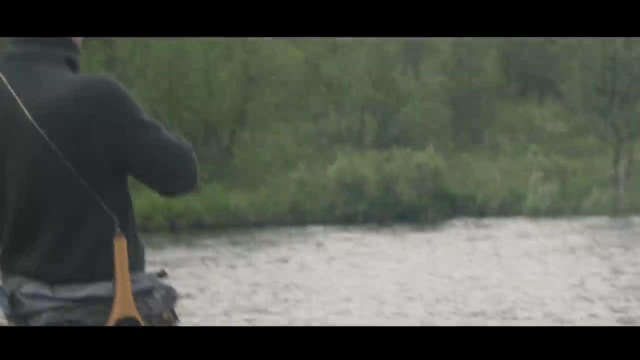 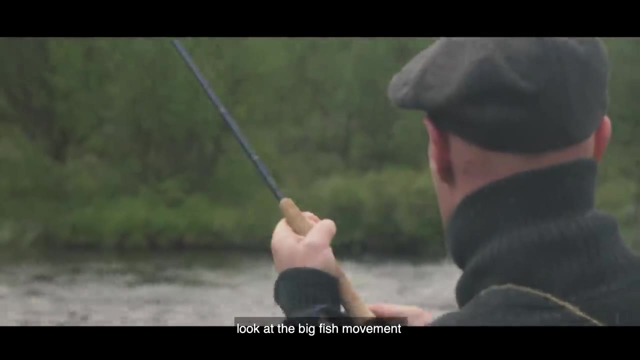 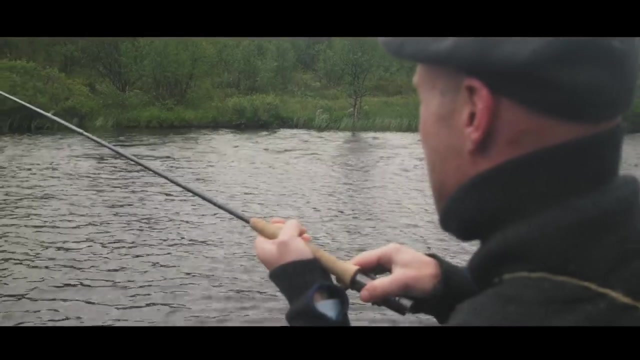 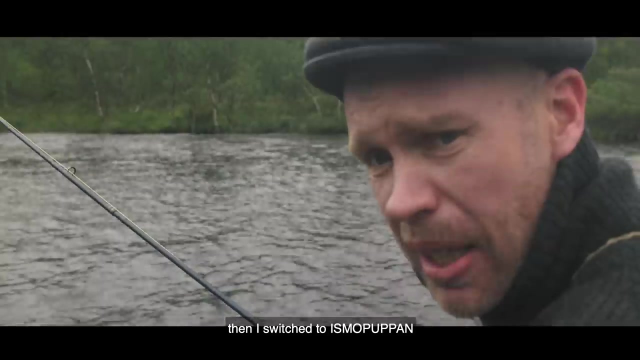 Yes, yes, yes, At least two. Can you see how it's moving, How heavy it's moving, How deep it's moving? I think it's three kilos. I have no chance of holding it, No chance. I'm so awake I'll switch to a smoke gun. 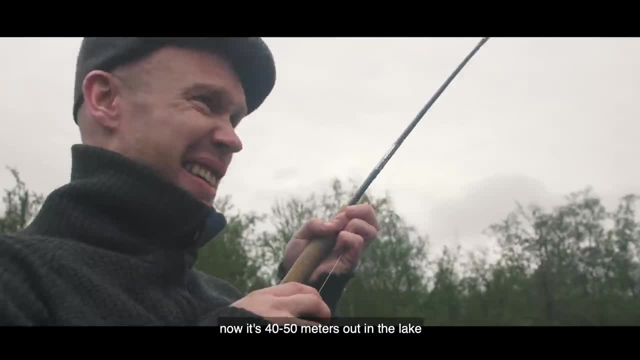 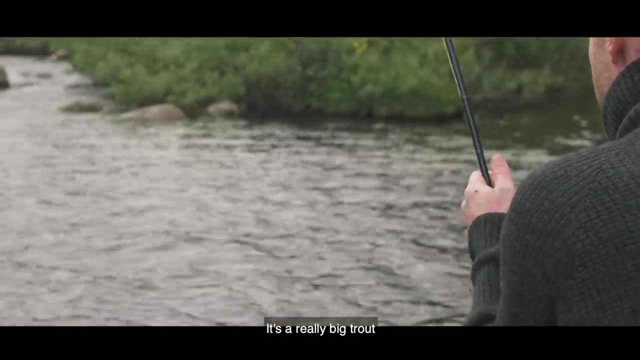 It took it right away. Now it's 40-50 meters out in the sea And it's moving, And it's moving. I don't know what else to say. It's a fucking big movement, But what the hell? It's as big as it is. 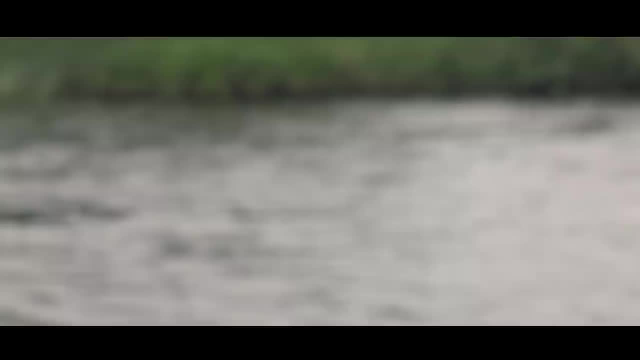 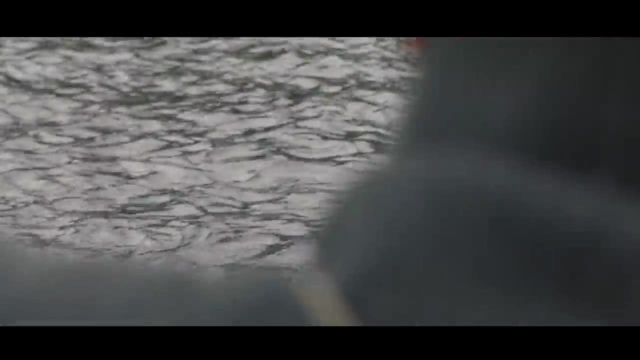 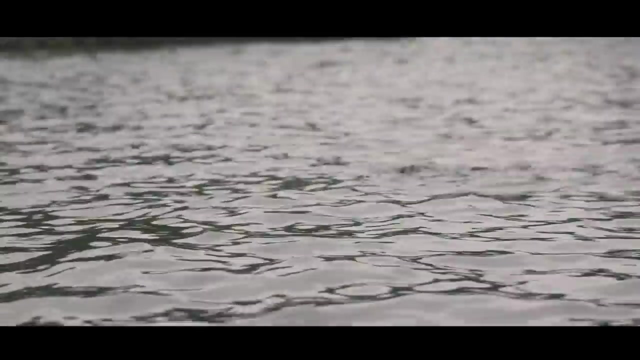 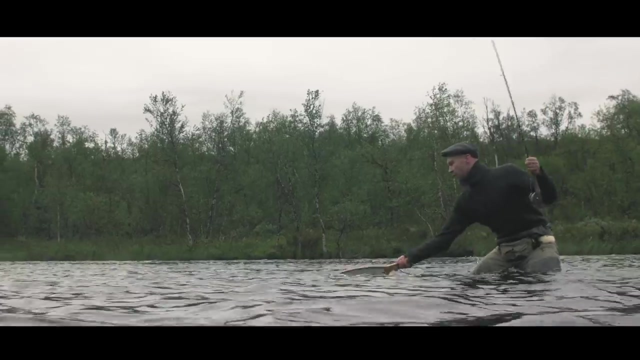 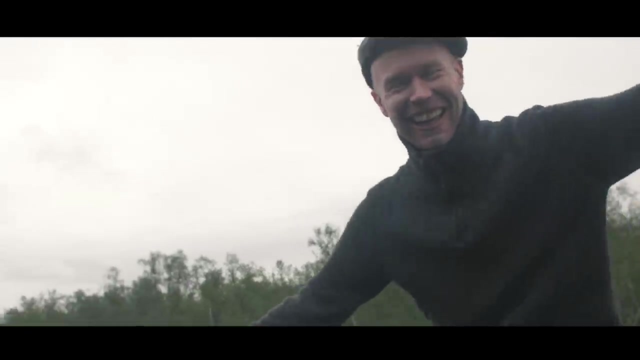 You can see it. What the fuck? I can see it, Yes, but it's mega big, What the fuck, Holy shit, Come, Come, Come, Come now, Yes, Yes, for fuck's sake, What the fuck. 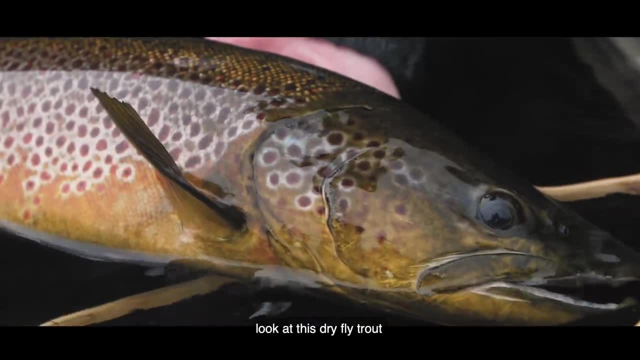 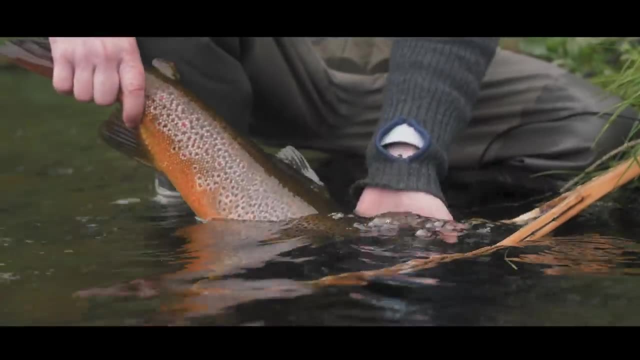 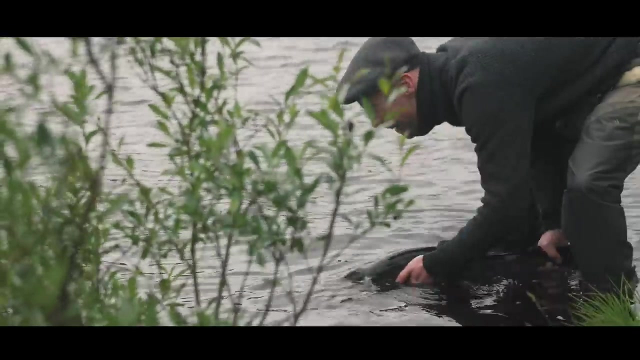 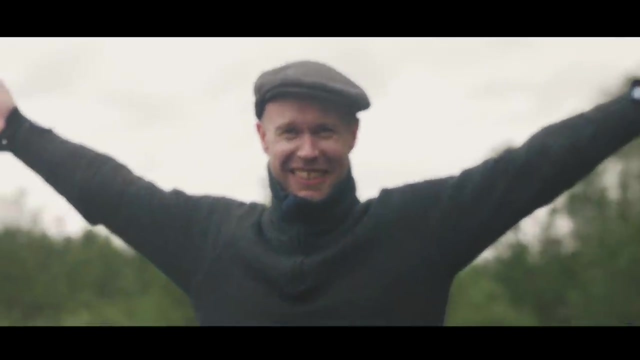 See: Look, a black-billed trout. Look at the black-billed trout. Look what kind of black-billed trout this is. What is that for something? What is that for something? Hovand was happy And I was happy for him. 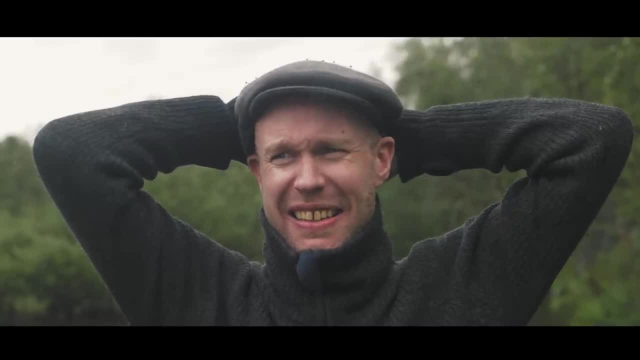 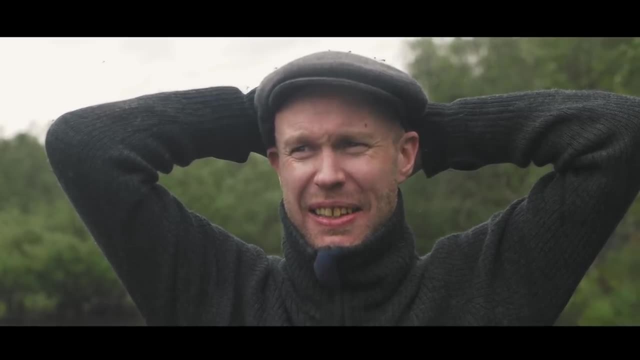 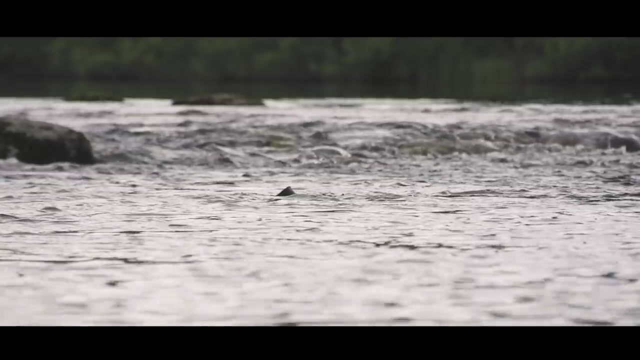 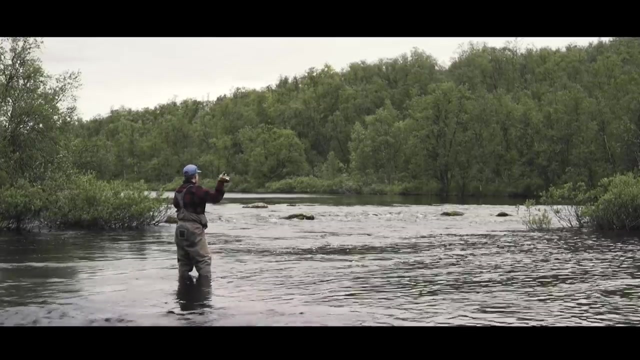 But I also felt a little seed of envy inside of me. I tried hard not to show anything, but insisted that we should go back to the pool where I had lost my trout earlier and it was back feeding. Perhaps Håvard and I could end the day as equals.